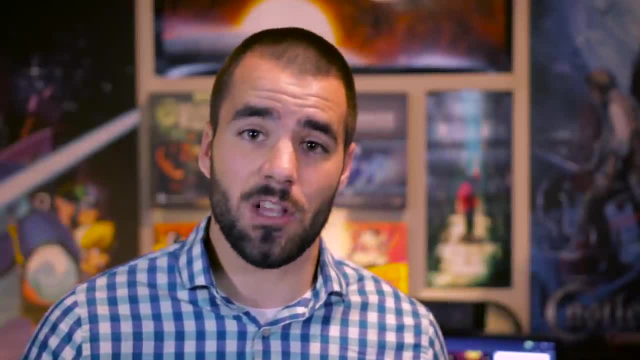 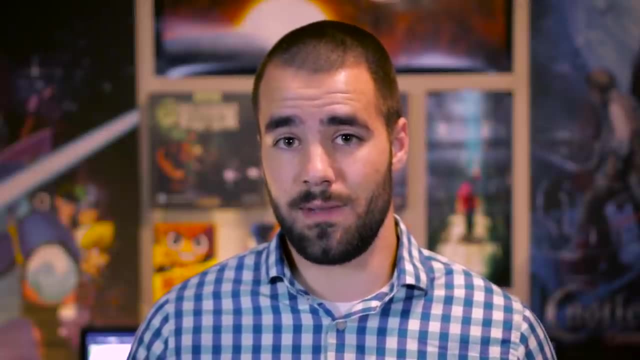 going to be able to contemplate what you've said and more easily follow along with what you're talking about. Also, your rate of speech isn't the only thing you can control to make your speech better. You can also employ strategic pauses to highlight certain points. Now there's 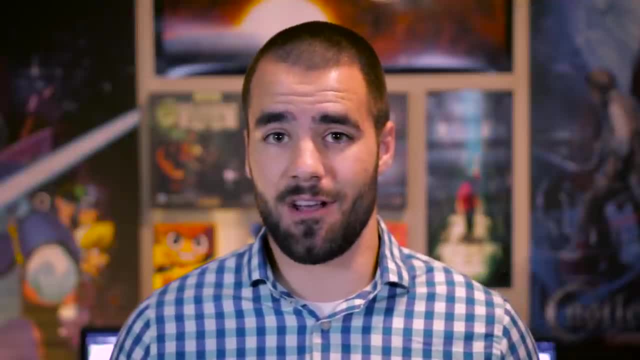 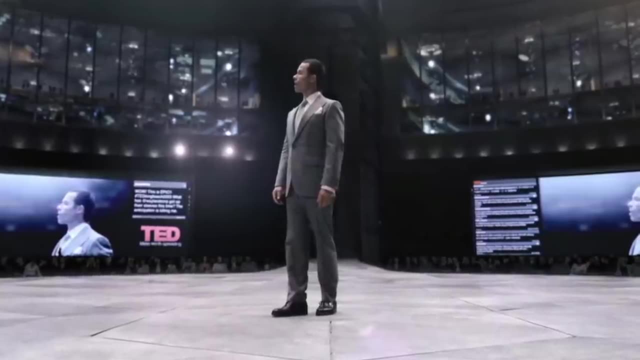 a lot of speeches that I've watched to study to become a better speaker myself, but there's actually a fake one that I really, really like and want to use as an example here, And it's this 2023 TED Talk that the producers of the movie Prometheus put out as an advertisement for the 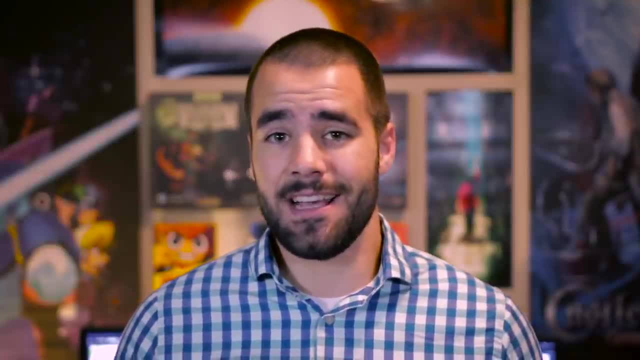 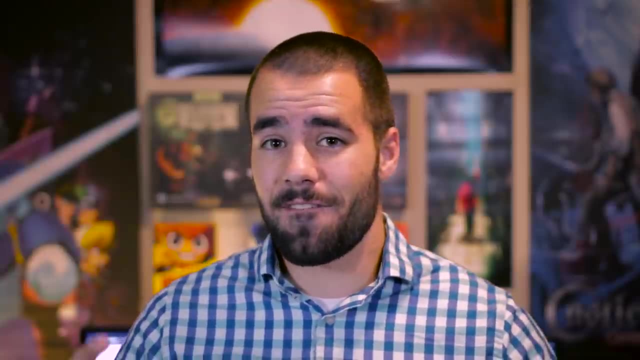 movie And in this TED Talk, Guy Pearce's character is talking about cybernetic individuals and basically his ambitions to take over the world. But when I watched this, I thought it was a fantastic piece to study for public speaking, because he employs these pauses so dramatically. 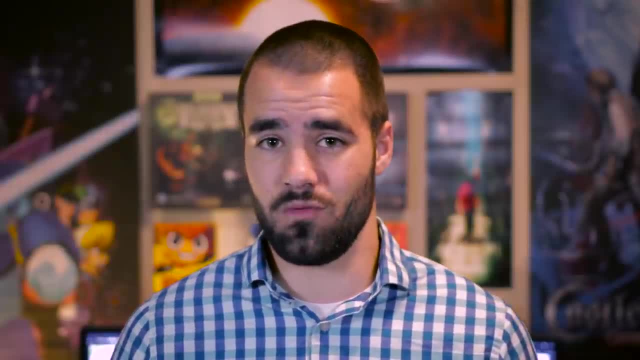 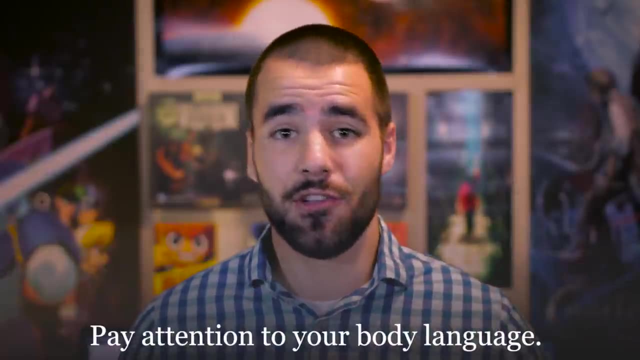 and so effectively. So check that video out after you watch this one. Now, another thing Guy Pearce does amazingly in that video is my second tip, which is to pay attention to your body language, And this is important for two specific reasons. Number 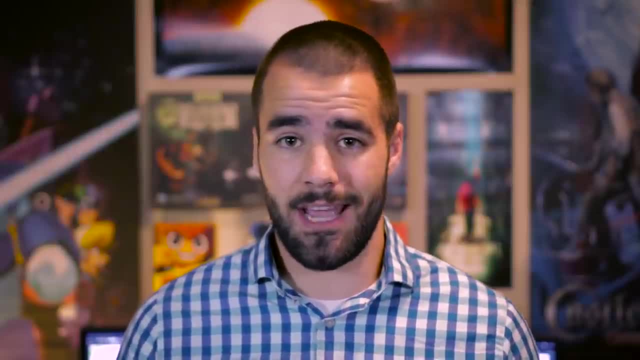 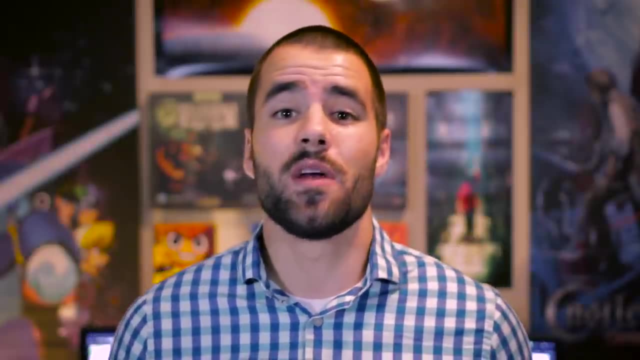 one. your body language forms a large part of the nonverbal communication that complements the verbal communication of your words: The way you hold yourself, the way you're poised, your posture, the way you move your hands and gesture to highlight certain points these. 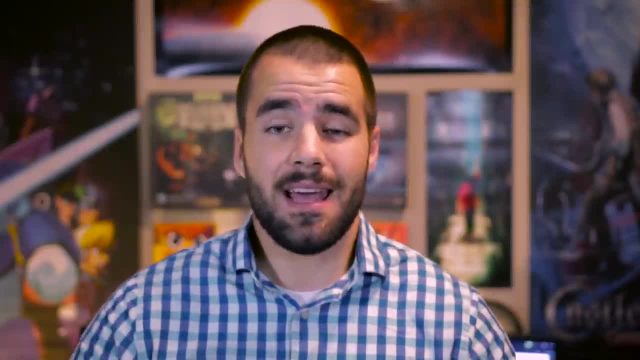 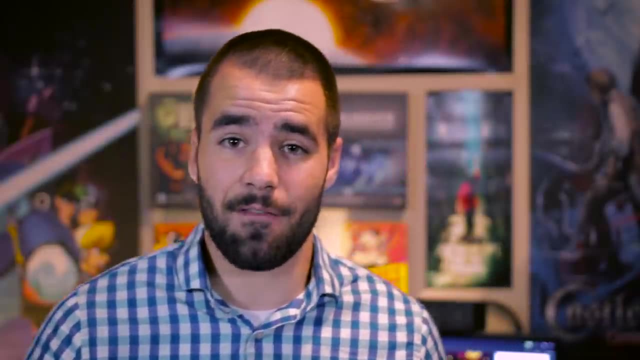 all go hand in hand with the words you're speaking and can help to complement and drive home those points. But the other reason is that the unconscious body language that a lot of inexperienced speakers have is something that can harm you. We have a lot of nervous tics, For example, when I was an inexperienced speaker just starting. 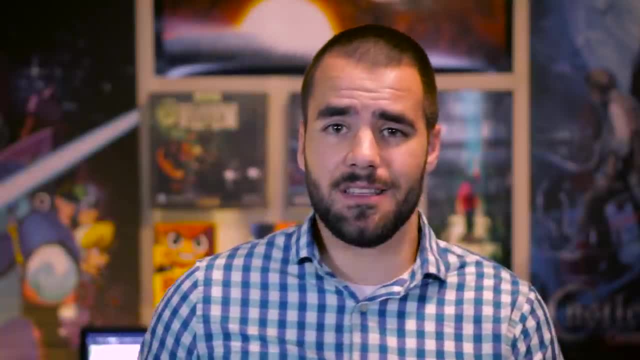 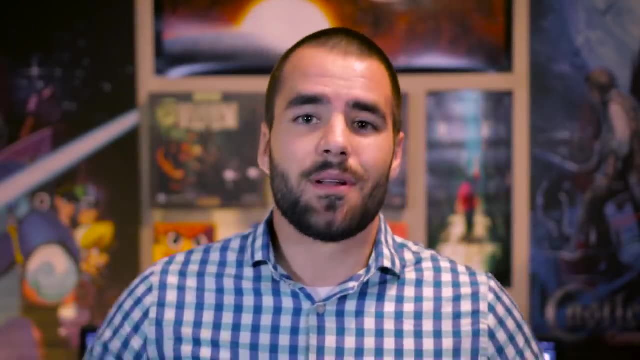 out a lot of things that I would do. I would put my hands in my pockets and I guess the camera's fixed right there, but I can try to show you right. I put my hands in and out of my pockets over and over again while I was speaking, And I would also pace around. 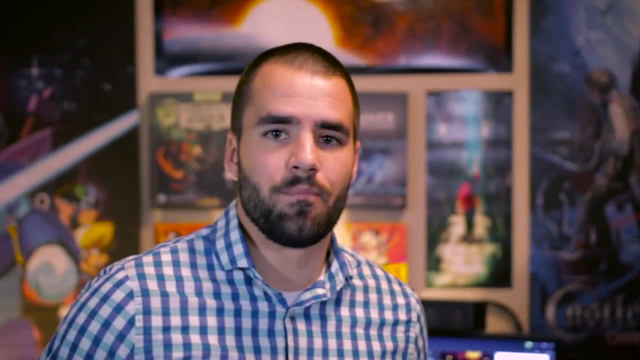 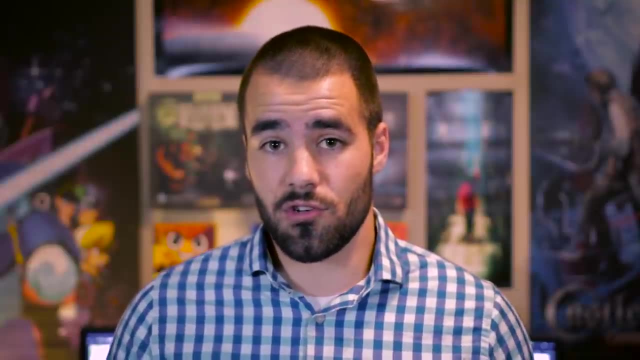 the stage really distractedly kind of moving And I wasn't really consciously pacing. I wasn't really pacing and using that to affect. I was just doing it unconsciously. So these are things that you can control to both not distract your audience but also to help bolster. 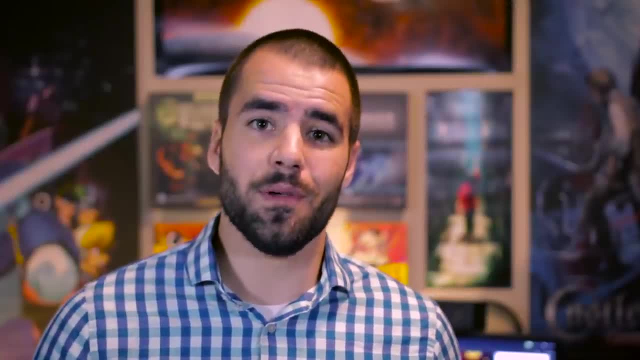 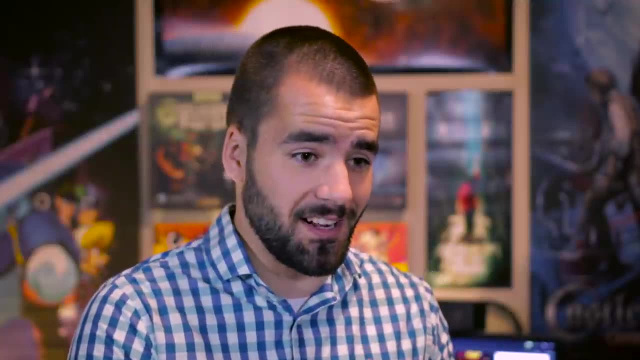 your points Now. my third tip is to consciously try to improve your ability to make eye contact with your entire audience. Now, one thing rookie speakers do a lot of times is they'll fixate on one section of the audience and they'll stay there during their entire speech, because 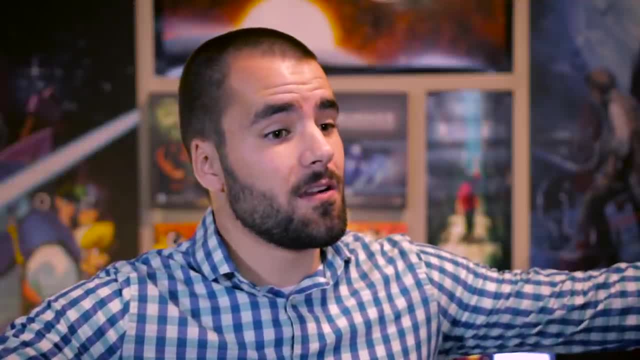 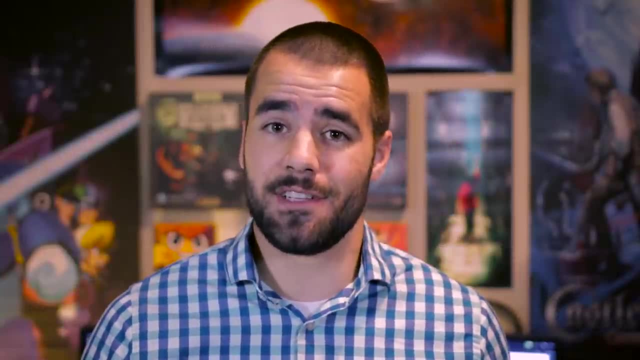 they're nervous. But the problem is there are people over here and over here and your entire audience are the people you're addressing, So you want to make sure you're trying to make eye contact with each and every single person during your speech. Now, I know it can be difficult to make eye contact when 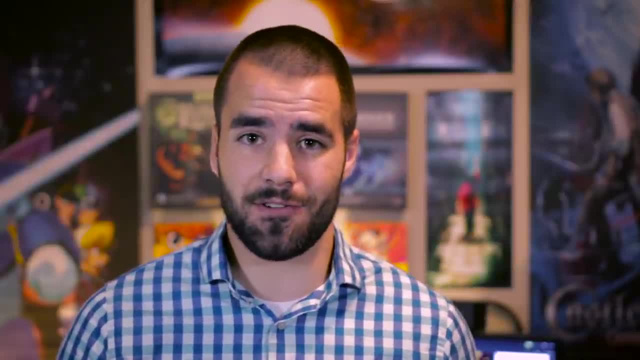 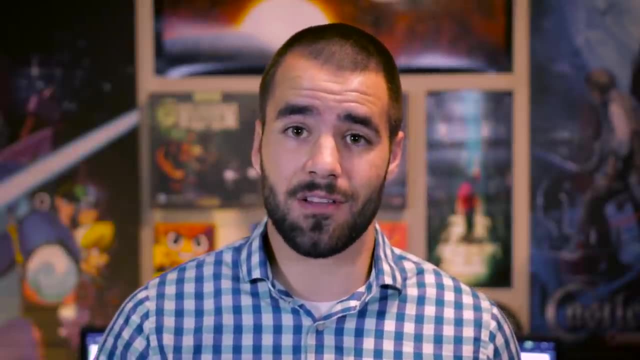 you're already nervous about being on stage, So you can employ a classic speaker's trick, which is to simply look over the heads of the people in the back row who are far enough away that they probably won't be able to tell that you're not looking them directly in the 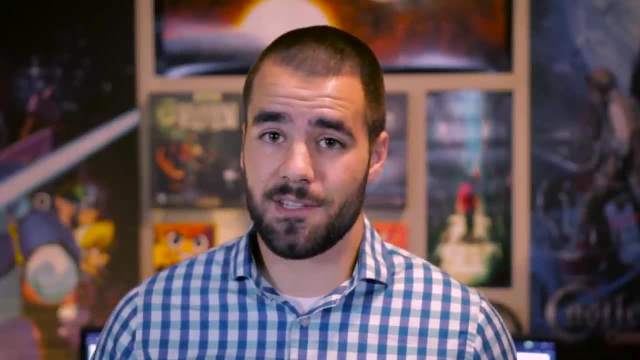 eye, But I do want to challenge you. The next time you have to make a speech, if you're feeling nervous and you find it difficult to make eye contact and you want to employ this trick, I do challenge you to at least try to make eye contact with your entire audience. 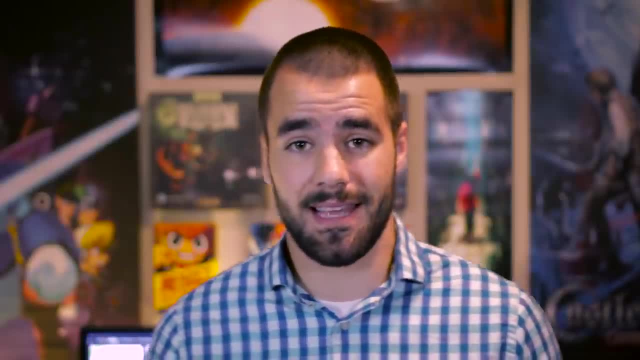 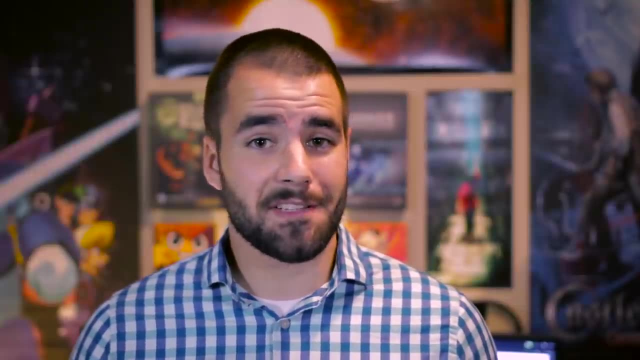 If you can't make eye contact with a couple of people throughout your talk, because this is something that gets easier to do over time and it will make you a more engaging, effective and more human speaker. Now, speaking of practicing that eye contact, the fourth tip is to in general practice. 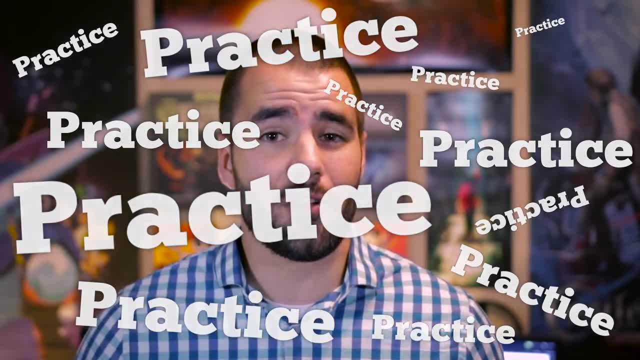 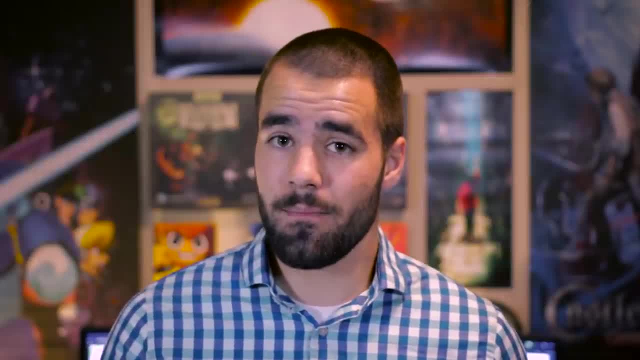 Practice, practice, practice, And when you think you have practiced all you could potentially ever practice, do it again. The idea here is not to practice your speech until you get it right, but to practice your speech until you can't get it wrong. And this is because 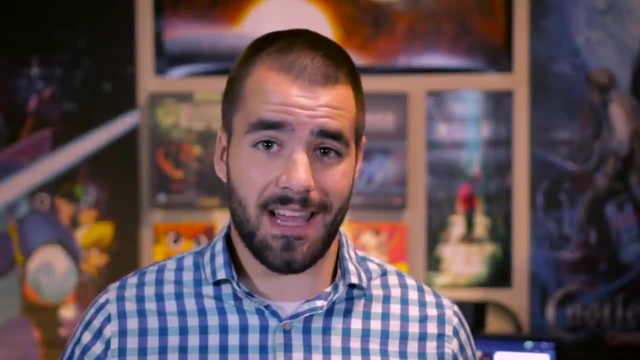 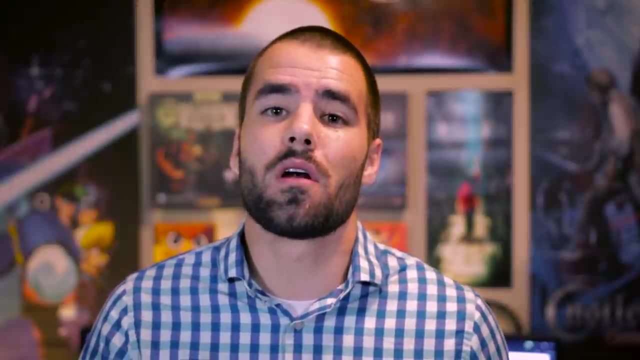 mastery helps to get you through any anxiety you're feeling. As we talked about in my test, anxiety, video anxiety can actually block your brain from making connections. So the more concrete grasp you have on your material, the more likely you're going to be able to. 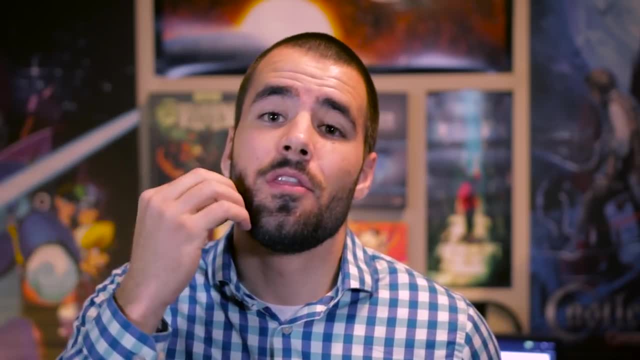 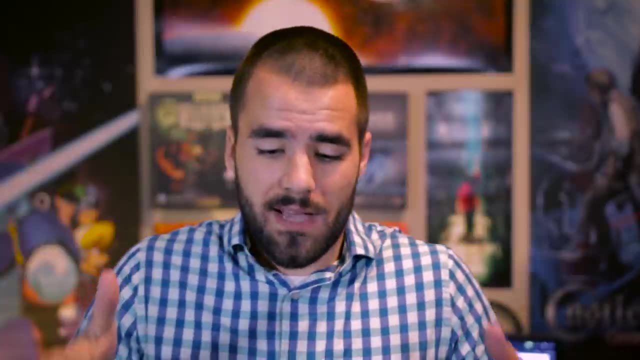 get past those anxiety blockers, get the thoughts out of your brain through your lips and into the ears of the eager audience. Also, mastery is important because when you're getting something right in your practice situation, it doesn't necessarily mean you're going to be able to. 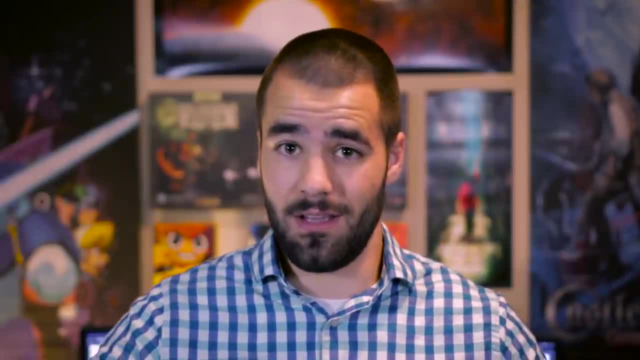 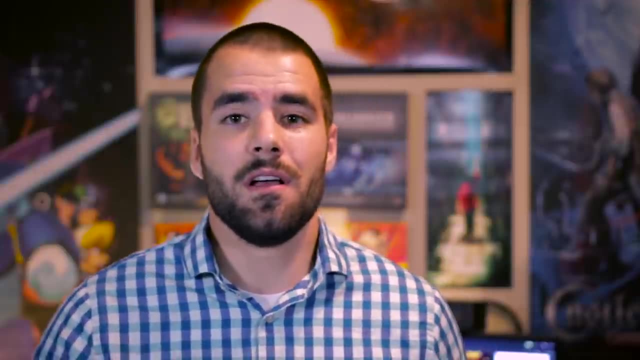 get it right in the more stressful situation where you're addressing real living, breathing, farting human beings right. So make sure you practice until you know your material cold Now. on that note, you might be thinking. well, my speech teacher told me not to memorize my speech. 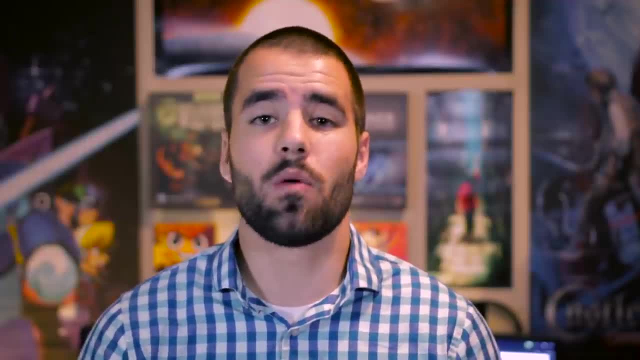 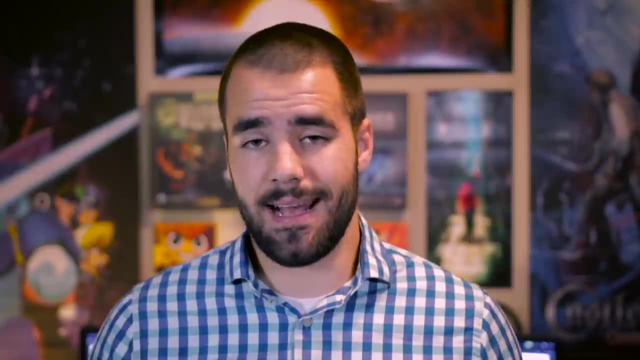 And in general I do agree with that piece of advice, but I want to drill into it and give a little bit more of a specific opinion on it. So in my mind, you should not write your speech out like an essay and try to memorize it word for word. If you do that, you're going to sound 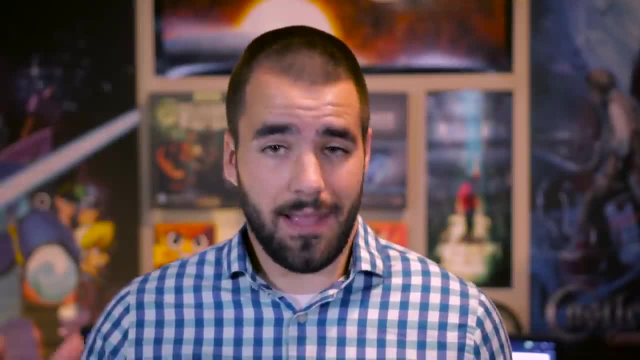 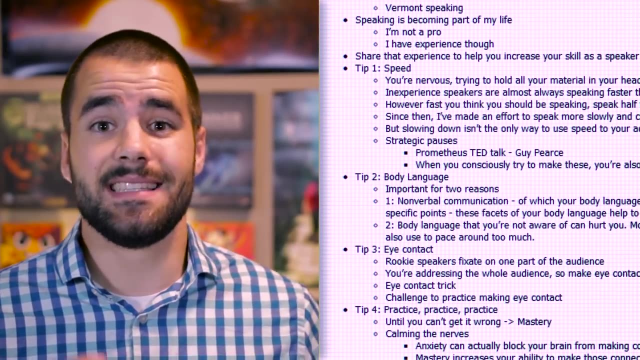 unnatural. You're going to sound robotic, You're going to sound like you're reading, But I do think you should write your speech out in the form of bullet points. have the main points listed out, have any details and facts and statistics and figures you want to cite written out and memorize. 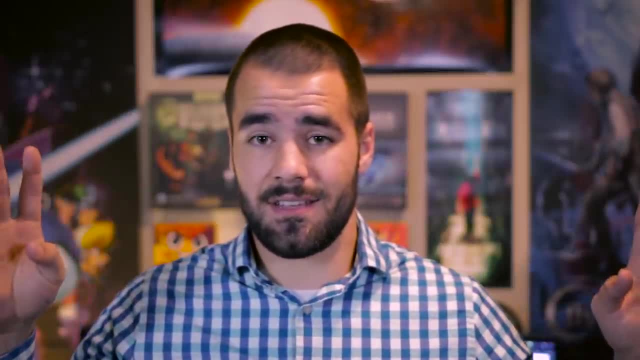 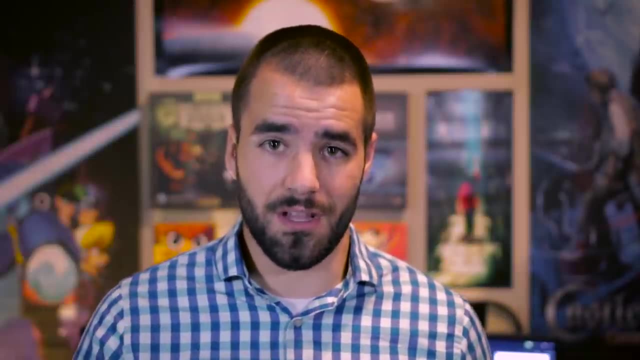 those. So when you get on stage, you don't have anything in your hands except maybe a presentation remote or a prop, And you can recite the entire speech from memory, because you know your points cold. You know exactly what it is that you need to communicate to your audience. 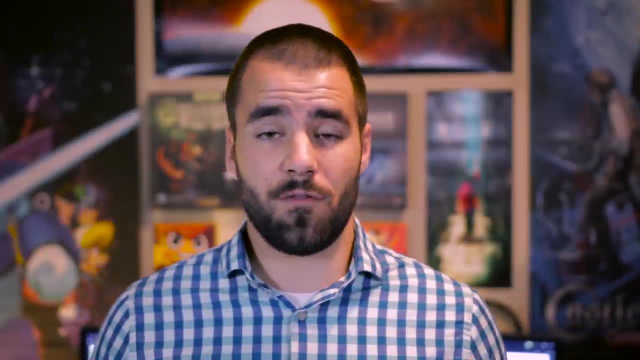 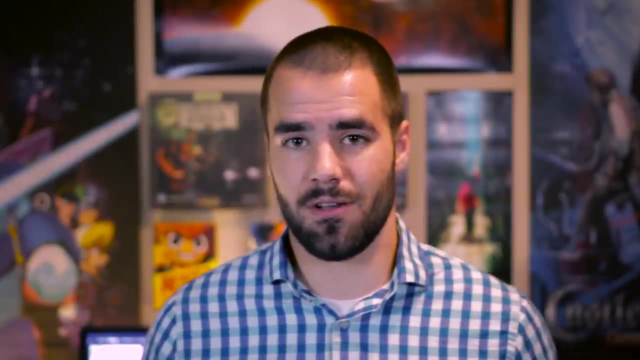 Now, another final note on practice is that practice works for individual speeches, but it's also something that's going to make you a better speaker over time. So if you feel like right now, your public speaking skills aren't at the level you want them to be, the best way to. 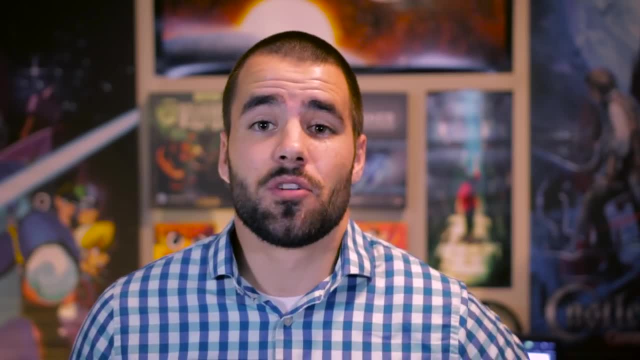 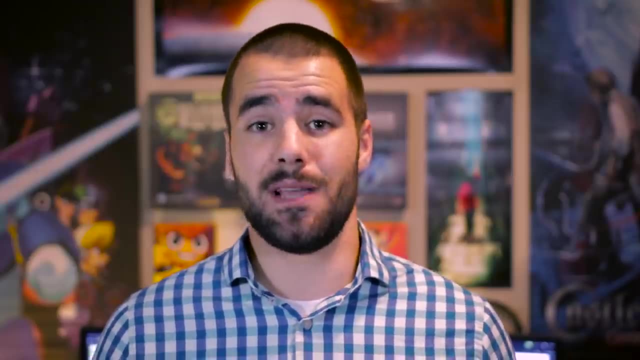 get better is to simply speak again and again and again. There's an organization called Toastmasters where you can get with other budding speakers and people who want to improve their skills and actually get up and give speeches. in a non-threatening environment You can take a speech. 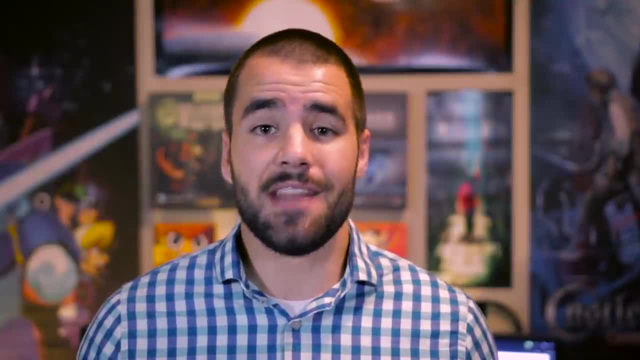 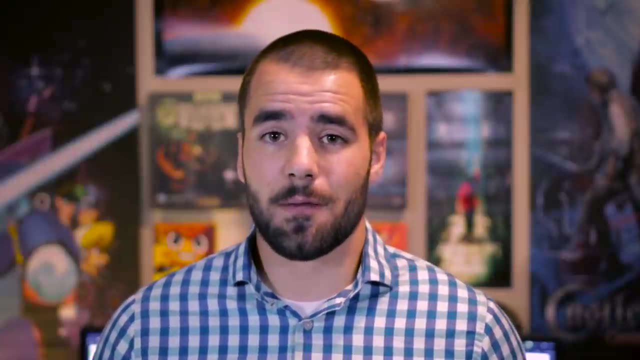 class at your school, which I definitely recommend you should do, And you can also do things that aren't really public speaking, but just things that give you performance anxiety. If I'm being honest, the thing that has helped me become a better public speaker the most is running my podcast and my YouTube channel, because each and every 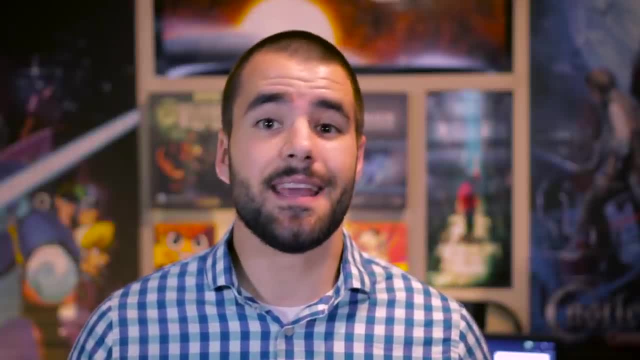 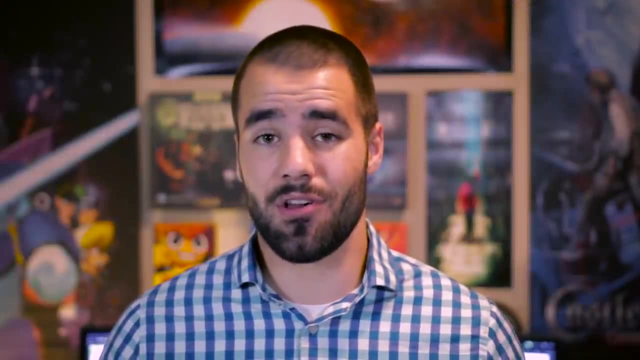 week, I have to create something where I'm speaking to an audience. Yes, my actual public speaking experiences have contributed to my skills, but I've done way more videos and way more podcasts and those have helped me as well. So if there's something that gives you performance anxiety, whether it be dancing in public or 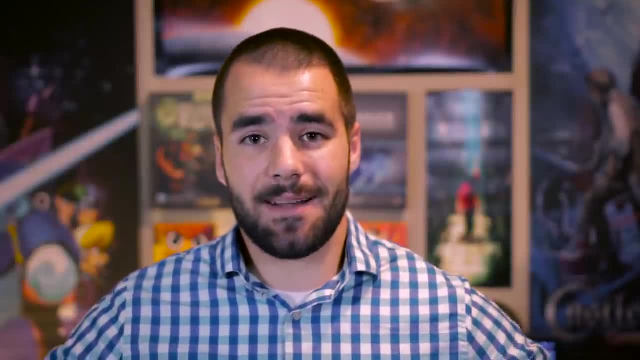 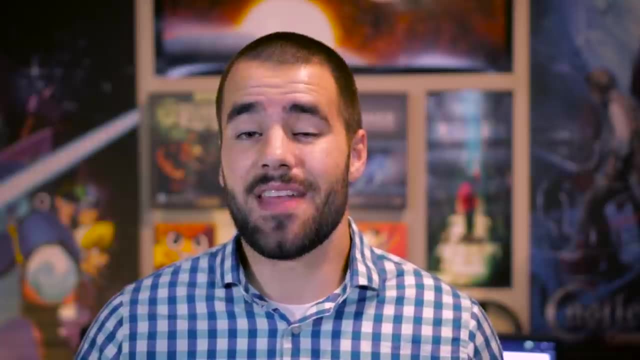 doing karaoke with your friends or something, anything that gives you a little bit of anxiety up front, but then afterwards you realize that the world didn't end, even though you did it. that's going to help build your confidence and decrease the amount of care you have for. 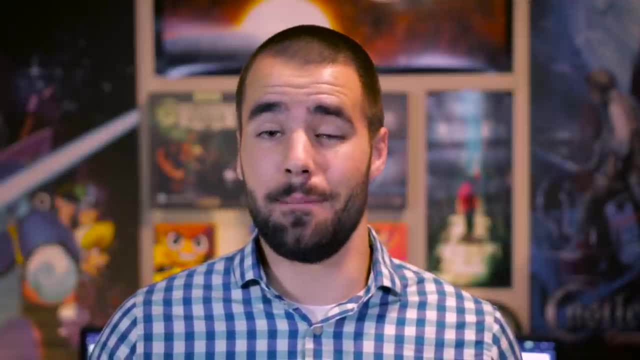 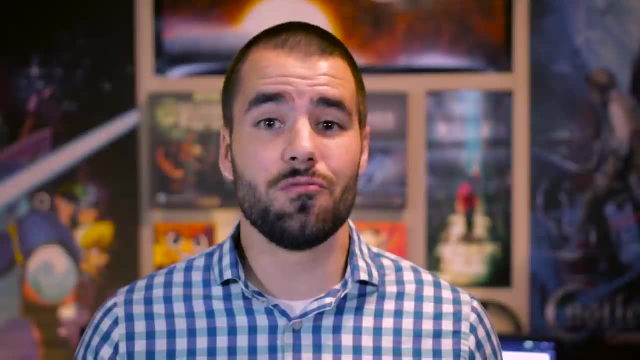 what people think, And those improvements will all feed back into your speaking ability. Now my fifth tip is also related to practice, but it's a little bit of a technical improvement you can make to your practice, and it's to do exactly what I'm doing right now, When 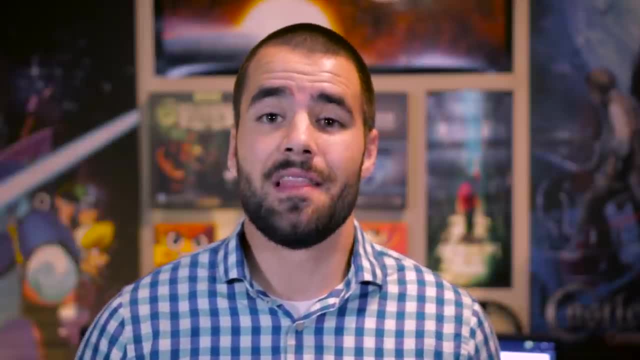 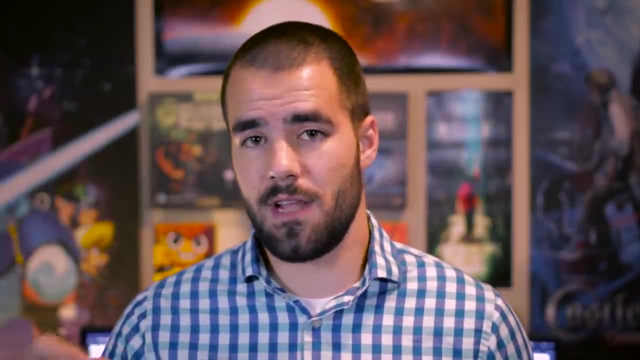 you practice, take a video camera with you. This is what I would do every single time I had a speech in college. I would go find an empty classroom and with my first few runs I wouldn't videotape it, because I was just trying to get the material down in my head. so I memorized it all. But once I had the 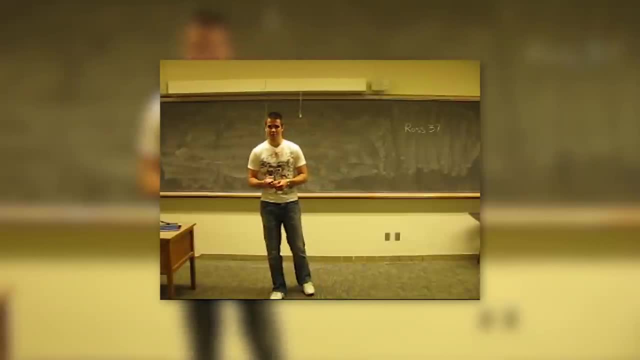 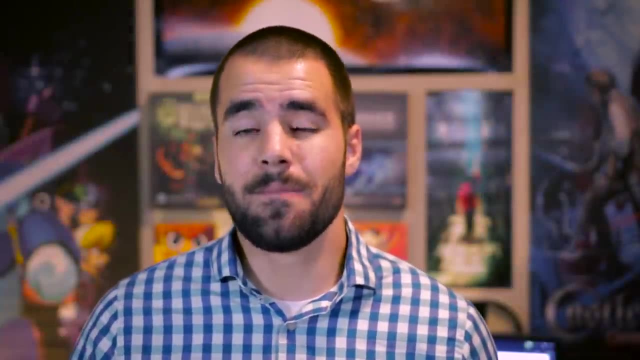 material down. then I would film myself doing each and every take And afterwards I would watch the take, review each aspect of my performance and pick out the things that could be improved. This is a huge upgrade over just practicing for an empty room, because you're not always. 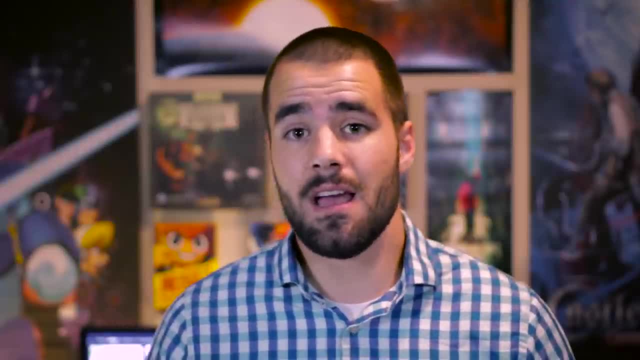 aware of the things that you're practicing. You're not always aware of the things that you're doing. Maybe you have a nervous tick, Maybe you're looking back at the slides too often, or maybe you're pacing too much, but the tape doesn't lie. So if you can watch, 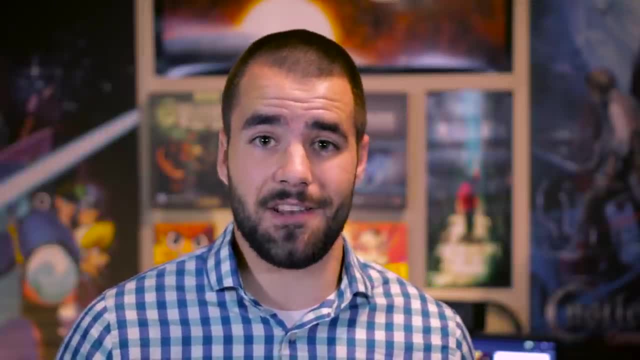 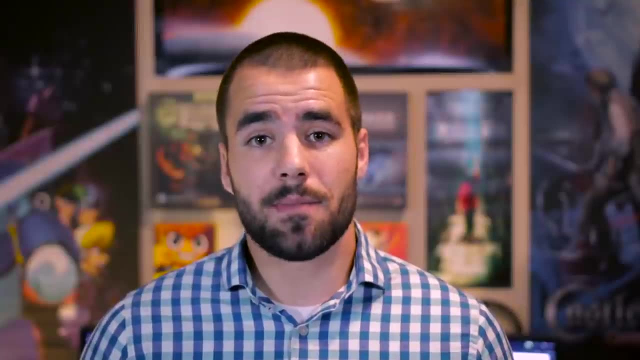 that tape, see your mistakes, you can know what to correct and you're going to be able to practice more effectively and maybe have to practice even less than you would originally need to. So tip number six is to know who your audience is, And by that I mean realize that people 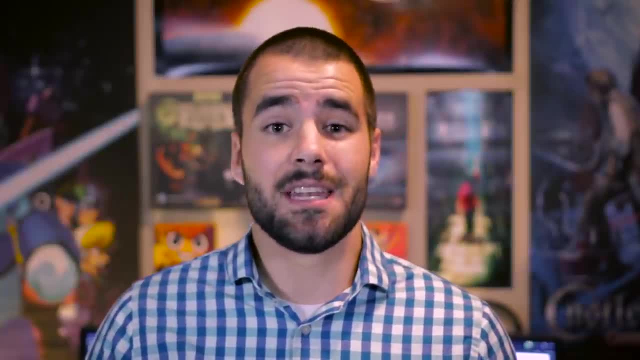 in your audience will most likely fall into one of two categories. Number one: over here you have the people who are the most likely to fall into one of two categories. Number two: you have the people who are rooting for you. They want to see you succeed. They're. 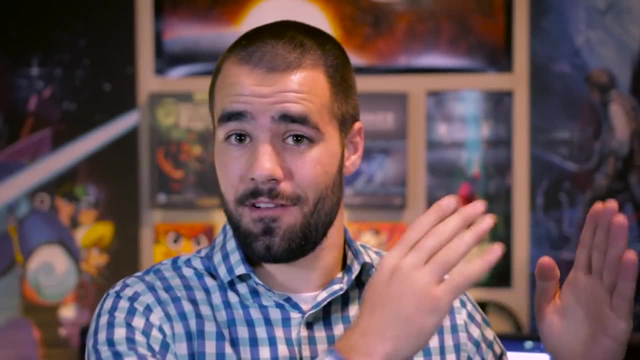 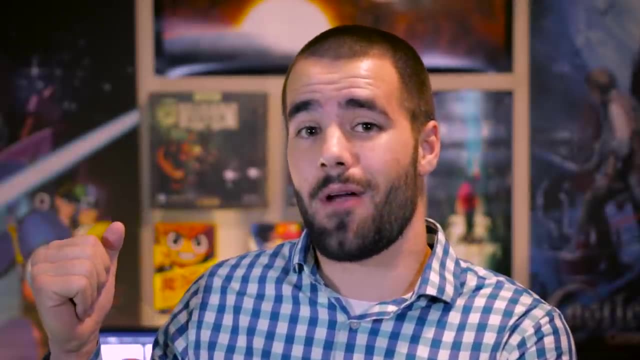 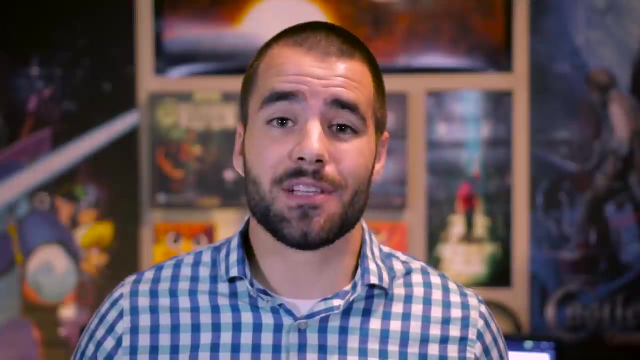 invested in your topic and these are your champions. like your fans, right And over here, you have the evil people who are going to laugh at you and throw tomatoes at you and curse your family for all eternity, right Or not. Over here, actually, you have people who are bored, and that's not because of you, It's. 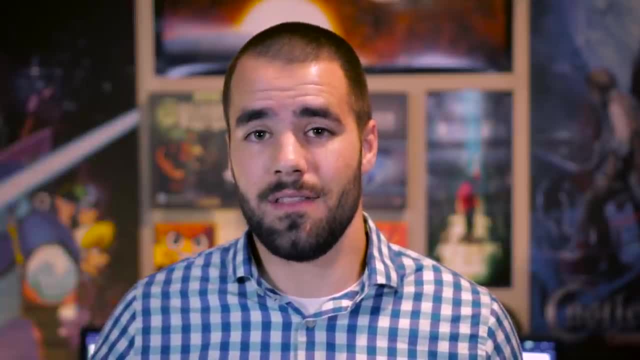 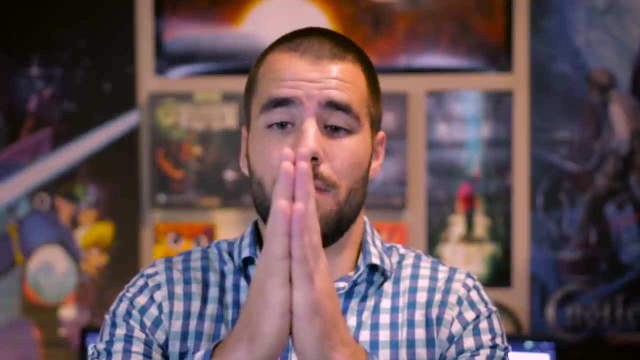 because their minds are elsewhere. They don't want to be there. They'd rather be off doing something else. And whatever you do- if you perform badly, if you perform really good or if you're more in the middle and just doing a mediocre job- it's likely that that's not. 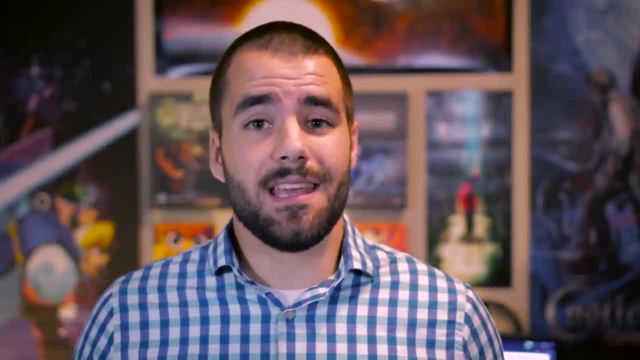 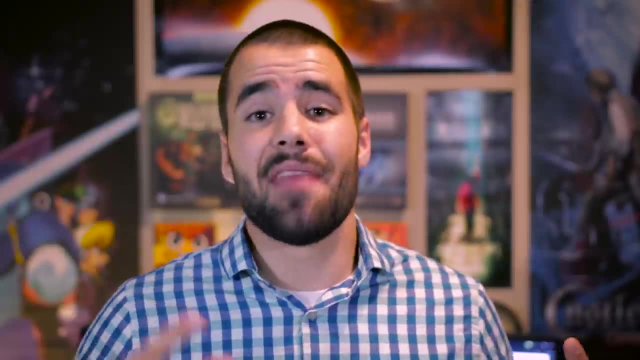 going to have much of an effect on them at all. Now, you do want to get the most number of people possible into that former category of the people who are really invested in your topic, And that's what the other tips in this video can help you do. But I want you to realize that the people in that latter category, the 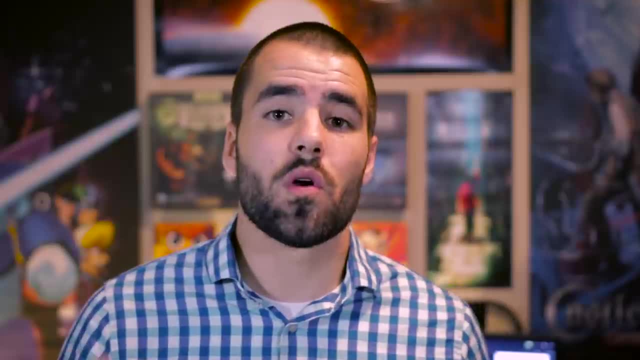 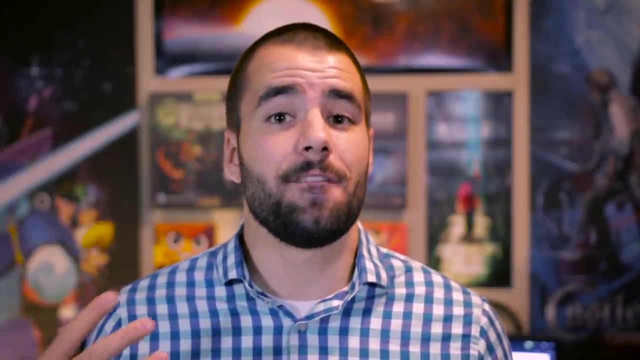 people who just don't care. they don't matter. So don't worry about what they're going to think when you're creating your speech or when you're up on stage delivering it, because that anxiety isn't worth it If you get feedback later on after the speech that you can use. 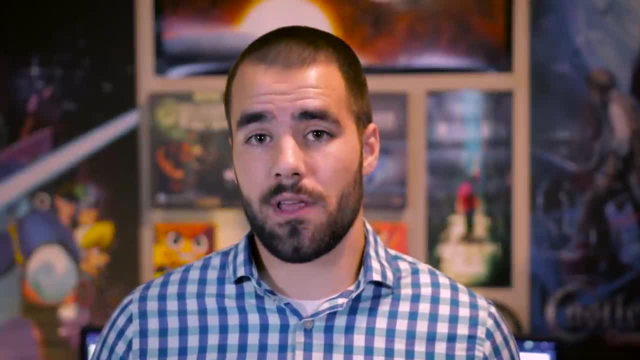 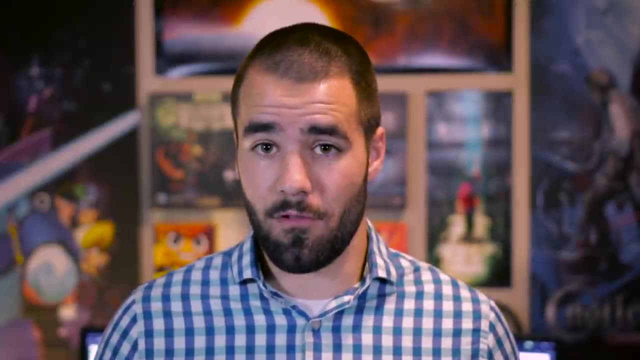 to constructively improve. that's good, but don't let it worry you in the moment Moving right along. my seventh tip is to focus more on the topic and less on the aspects of your performance when you're delivering your speech and also when you're preparing. 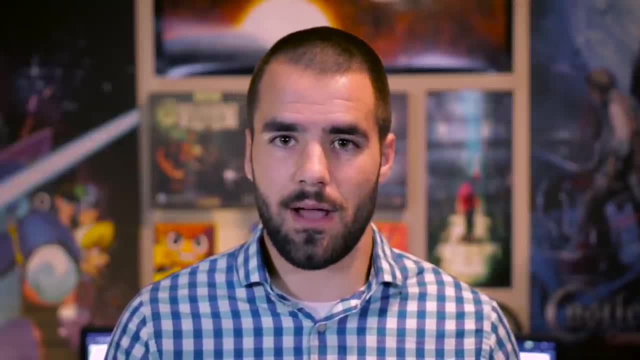 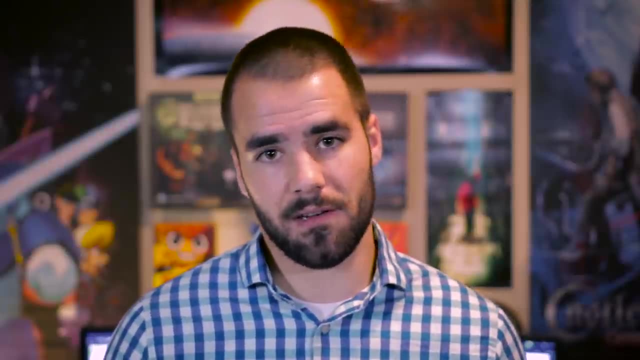 I found through experience that when I'm really invested in what I'm talking about and, more specifically, when I'm invested in a transformation I wanted to have on the audience, I don't care so much about that. I don't care about the technical aspects of my speech. I don't care about my body language. 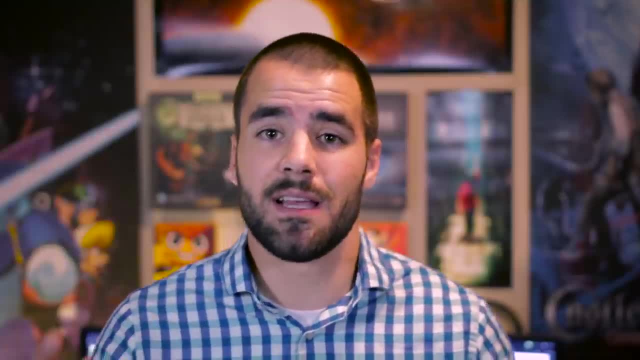 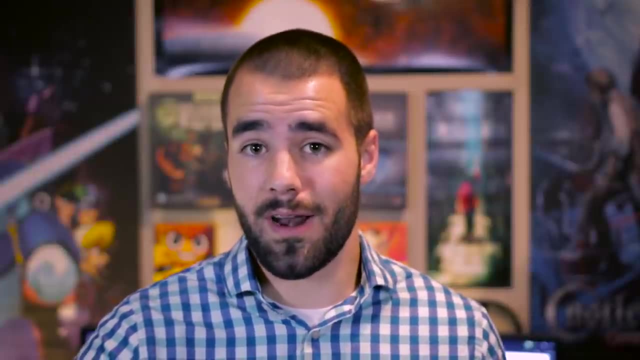 I don't care about my eye contact, I'm not even thinking about it, because it's become almost as if I was explaining something I cared about to a dear friend, and I want them to learn what it is that I know. So the focus comes off the nervousness of standing on stage. 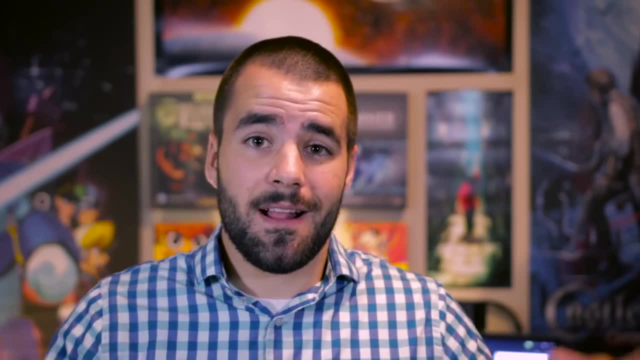 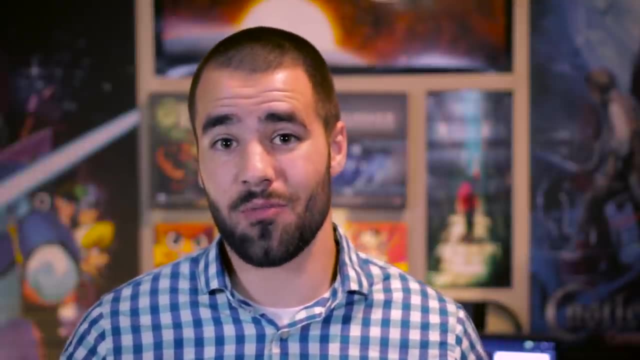 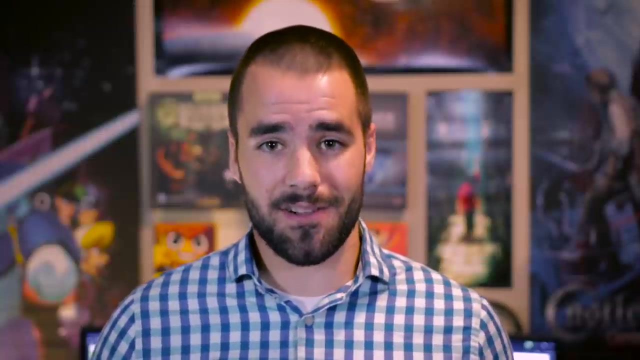 and addressing a bunch of people, and it's placed on. this is what I know and this is what I really want you to learn. I'm really excited about it and I hope that what I say makes you, or persuade you, to take some action. Tip number eight: don't have a stupid haircut. What I mean by that is think about your appearance. 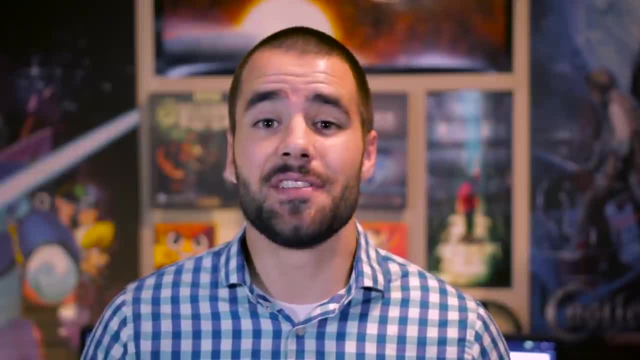 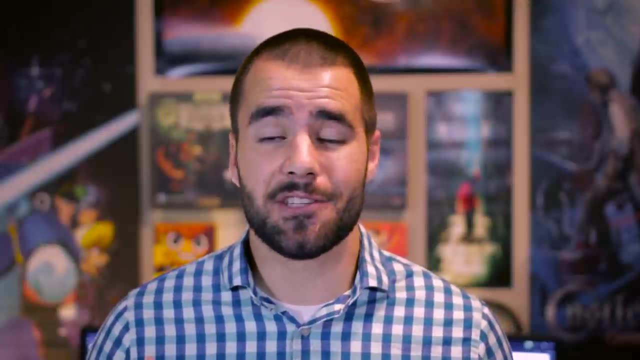 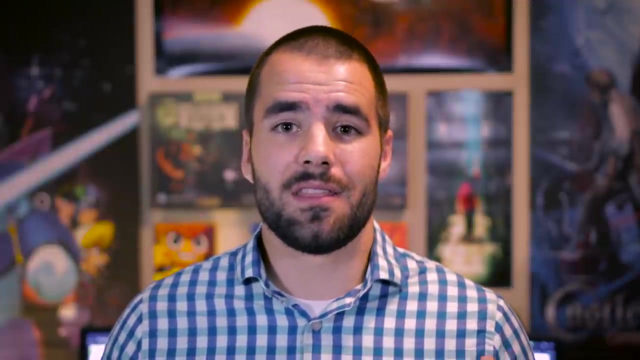 dress well and try to make a great first impression when you step on stage. This is important because of the halo effect, which is also known as exaggerated emotional coherence, and it's basically a term to explain the fact that humans make split second first impressions of people right when they meet them. So the problem with this is that maybe it's not a 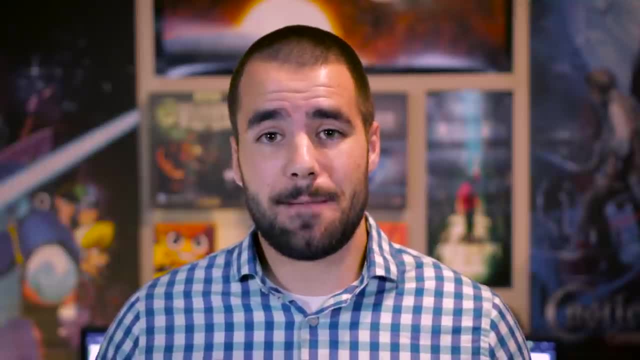 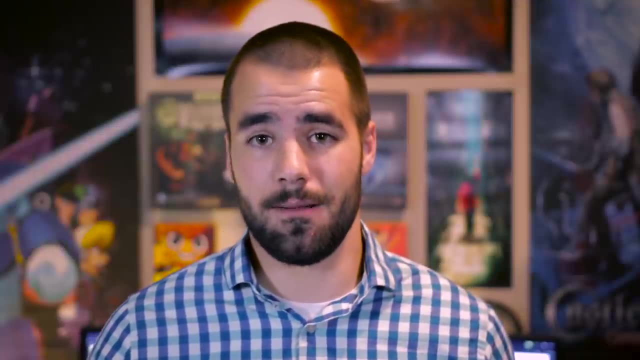 problem. Maybe it's just a fact of life. What happens is people use those first impressions to essentially fill in what they don't know about the person and also make judgments about what comes next. So if you get on stage and you're dressed well, you hold yourself well and people are. 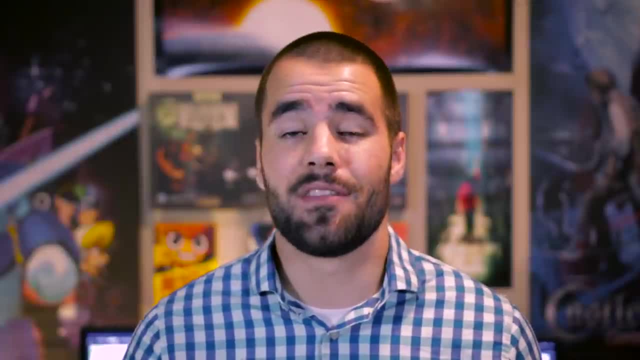 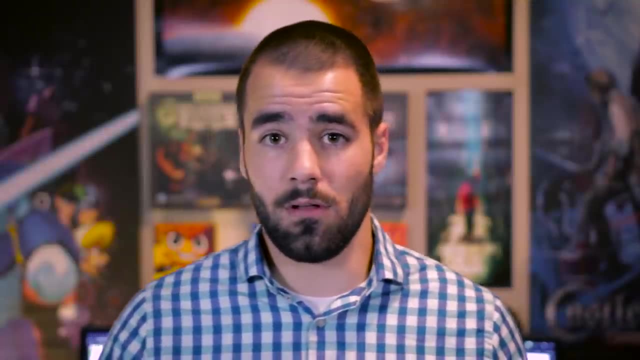 impressed with you, then they're more likely to forgive any mistakes you make and they're also more likely to be receptive to whatever it is you're saying. But if you don't look good, then it's going to be a lot harder for you to convince people of what you're talking. 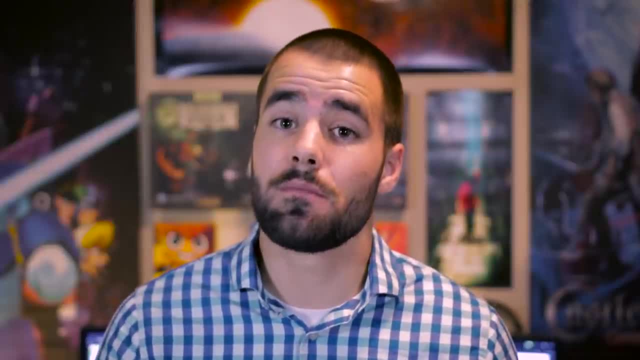 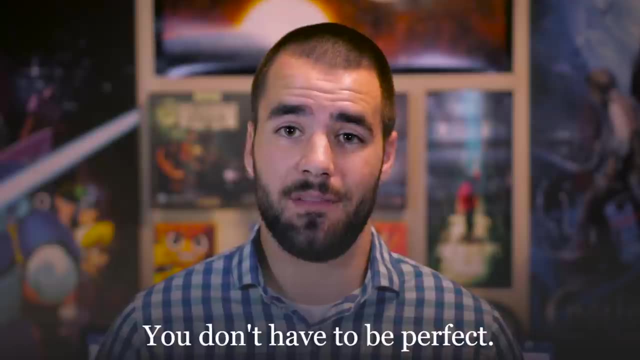 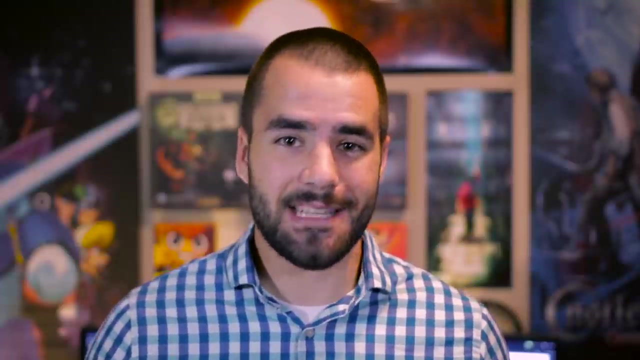 about and those mistakes will be all the more glaring. So first impressions matter And the final tip is… Take a breath, Don't think you need to be perfect. Focusing on perfection is the number one way to trip yourself up, to give yourself massive amounts of anxiety. 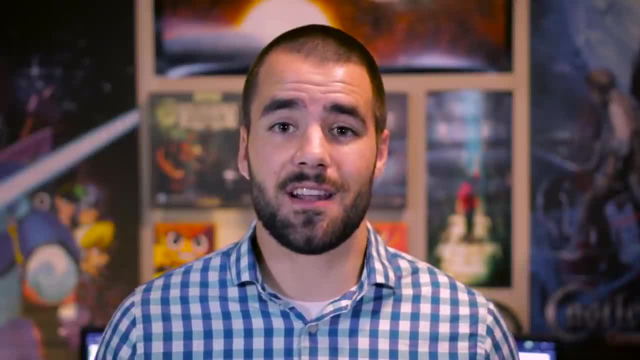 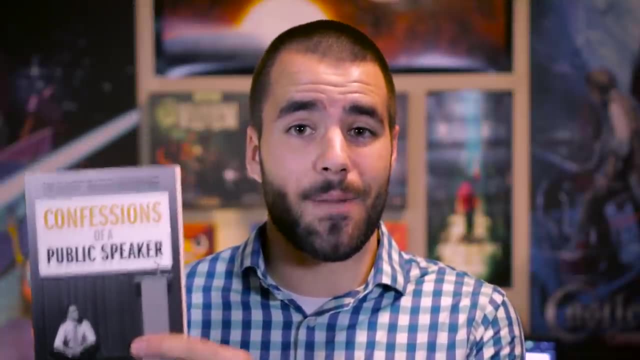 and to fail. Don't worry about being perfect, Just get on stage and deliver the best speech that you can give. There's a book I read in college called Confessions of a Public Speaker by a guy named Scott Birkin, and I highly recommend it. If you want to get better at speaking, it's on my essential. 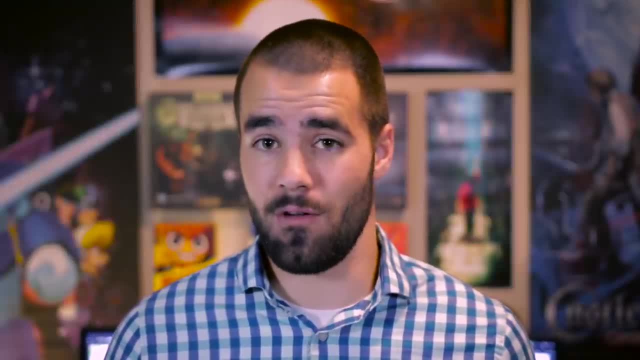 books list. But there's a passage in here that really resonated with me when I read it, And he says: I don't want to be perfect, I want to be useful, I want to be good And I want to sound like myself. 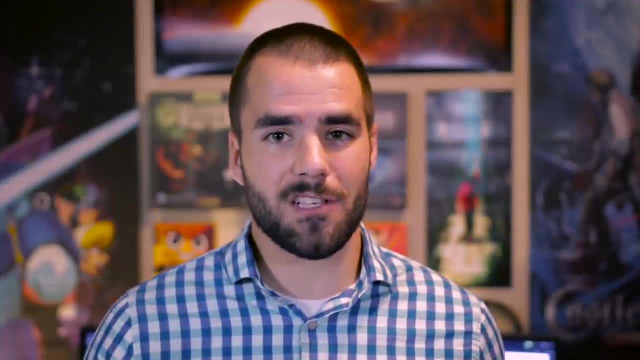 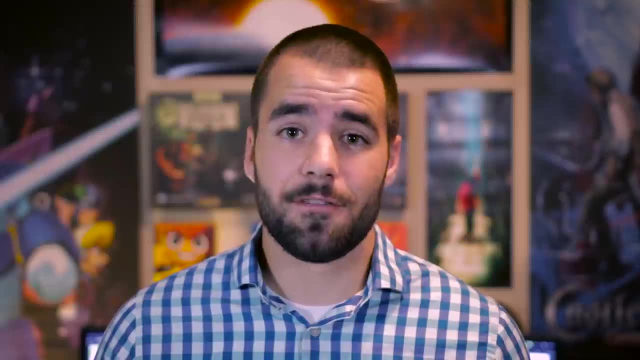 Nobody gives a perfect speech. Even if you think somebody gave a perfect speech, that person can point out all the errors and all the things they wish they would have done better. So get on stage, focus on doing good, focus on improving over your previous performance. 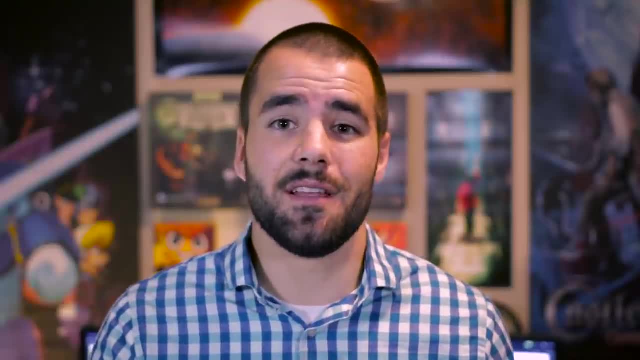 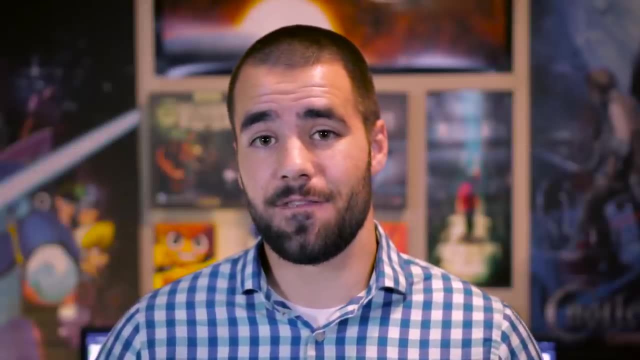 and then just focus on that topic. Like I said, try to enact a transformation in your audience and you're not going to care so much about your nerves and your performance. So those are the nine tips I wrote down for this video, But I do have a little bonus tip of sorts for you, and it's to study people who are 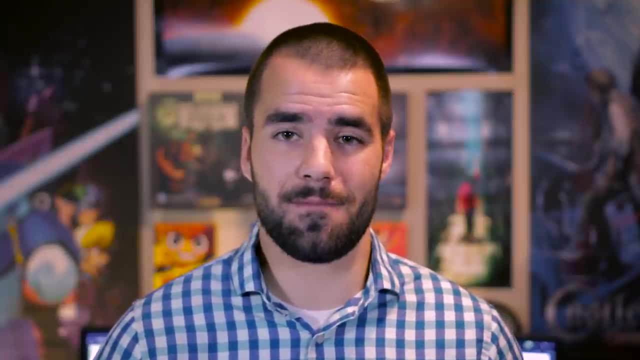 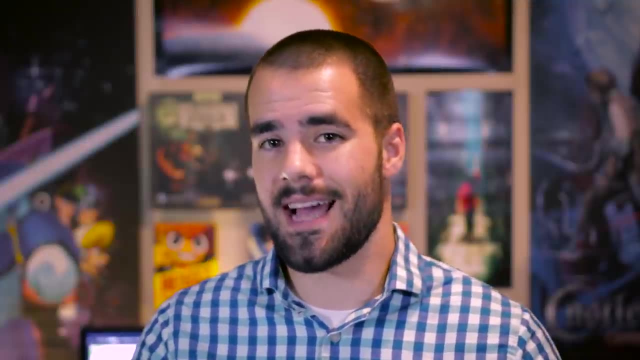 great public speakers. I have a playlist of videos here on YouTube that I've been building for a few years And whenever I need to make a speech of my own, I'll go study some of those speeches and try to pinpoint exactly what they're doing that I'd like to improve on with my 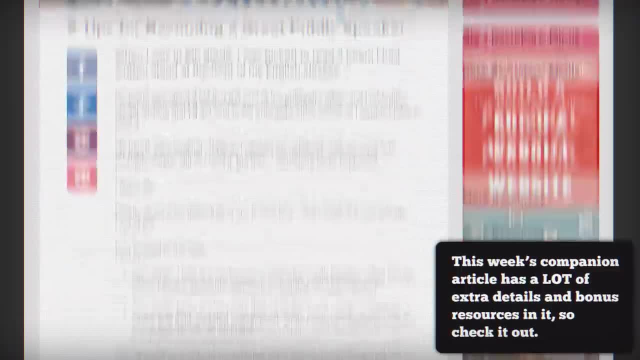 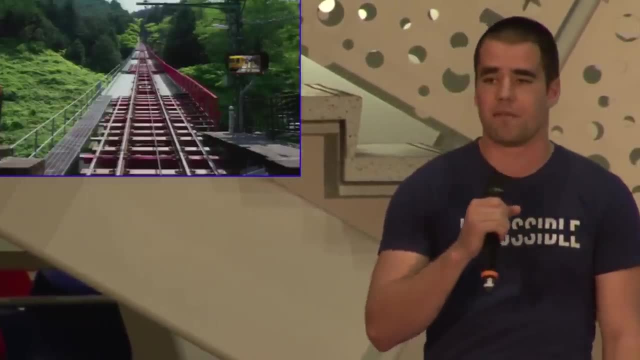 own skills. So in the companion blog post for this video I've linked to that playlist And as a bonus I've also linked to some of my earlier speaking videos. And just to forewarn you, one of the earlier ones is really, really bad. 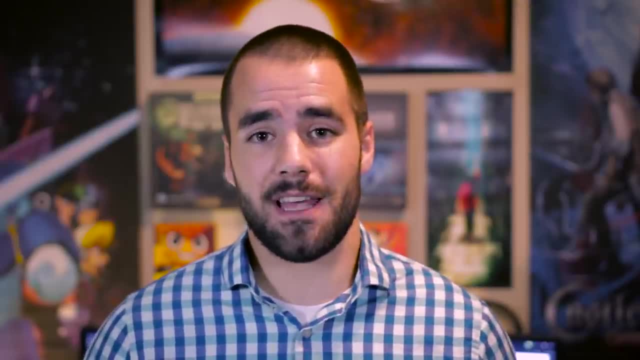 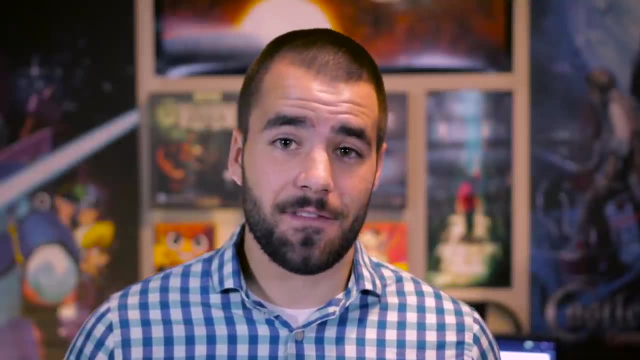 So laugh at me all you want, I don't care, because I have improved, And I just kind of want to show you guys that practice does make better, not perfect. So that's it for this video. Hopefully it helped you out, And if it did, I just want to let you know that next week we're going to follow up this.